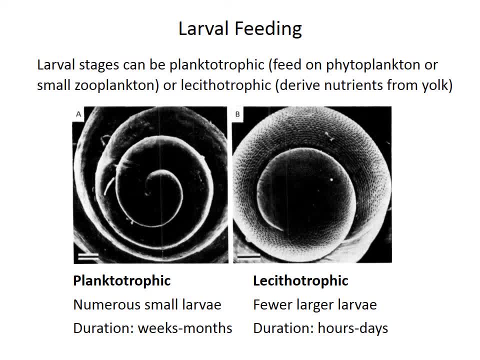 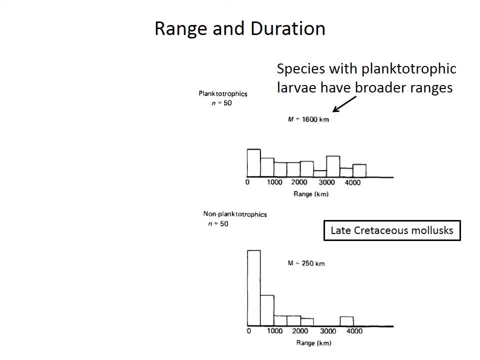 Leucithotrophic larvae, in contrast, settle within hours to days because they're constrained by the energy available from the yolk. Those differences in the nutrient source and especially in the time until settling, have important consequences for the geographic range and geological duration of a species. 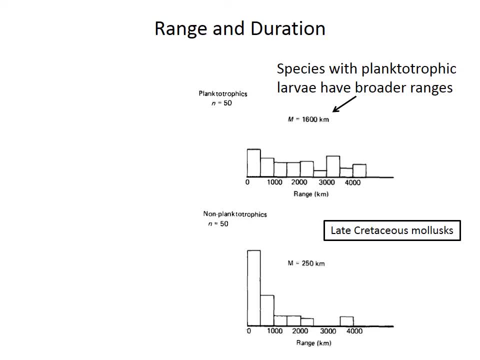 In this example from late Cretaceous mollusks, species with planktotrophic larvae have larger geographic ranges- on average 1,600 km, compared to only 250 km for the leucithotrophic species- Because of those range differences, 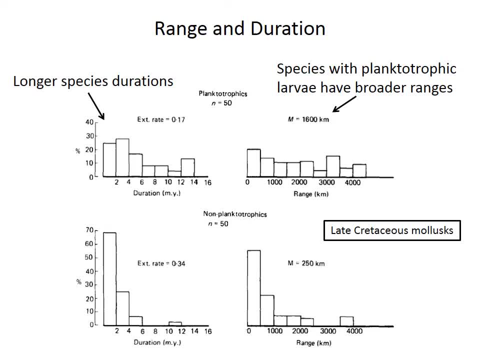 planktotrophic species also have longer geological durations. As you can see from the lower left panel, the non-planktotrophic or leucithotrophic species rarely persist longer than 2 million years in the geological record and they have extinction rates that are twice as high. 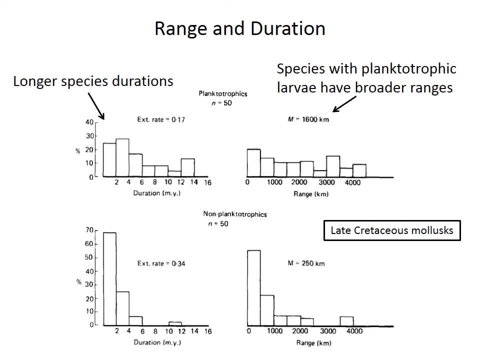 on average as the planktotrophic species. The relationship between smaller range and greater extinction risk arises in large part because narrowly distributed species can be more likely to be wiped out by chance events, whereas species with a broad distribution are going to contain subpopulations that have different tolerances. 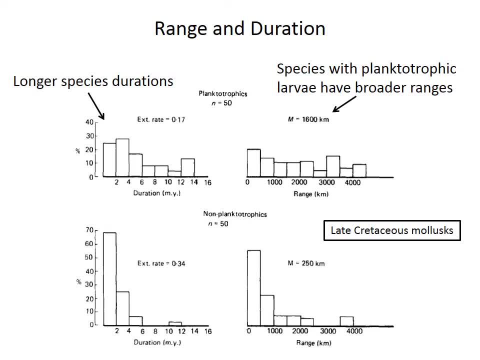 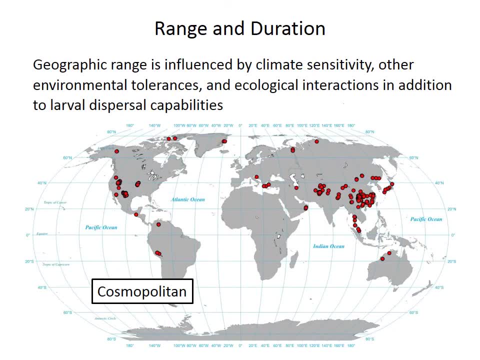 for environmental conditions and some of those subpopulations are going to be more adapted to dealing with or surviving in geological conditions. These subpopulations are going to be more likely to be affected by environmental changes. Larval dispersal capabilities are important influences. 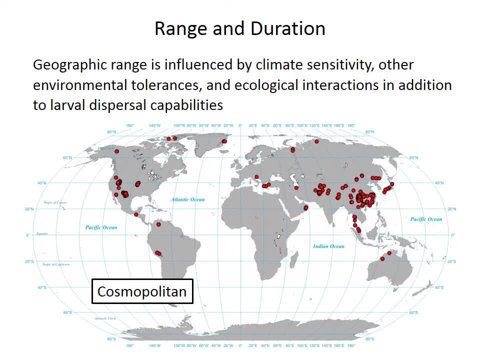 on the geographic range of a species, but they're not the only control. Climate sensitivity or other environmental tolerances, as well as ecological interactions, also control the distribution of a species. So there's two important terms to remember that can be used to describe a species distribution. 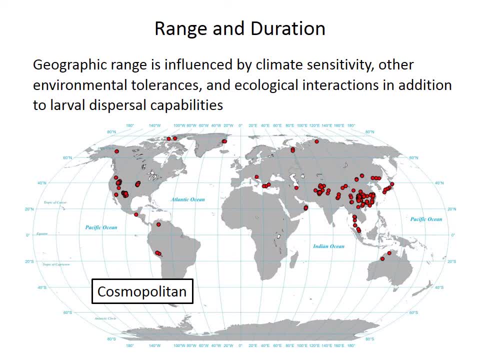 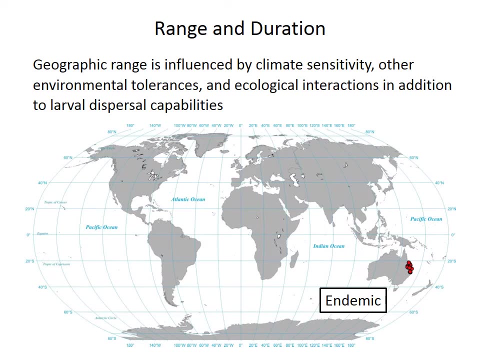 Species with a wide distribution, such as this one here. this example- these red dots reflecting the locations in which a species has been found- can be called cosmopolitan, whereas endemic species, such as this one here, are restricted to a small and localized region. 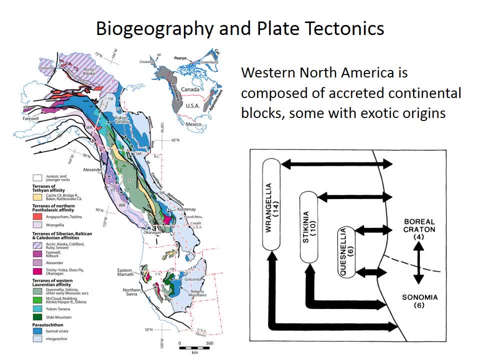 So one really cool application of paleobiogeography is in plate tectonic reconstruction, For example. much of western North America is composed today of accreted continental blocks called terrains. Some of those terrains appear to have formed pretty far from their current position. 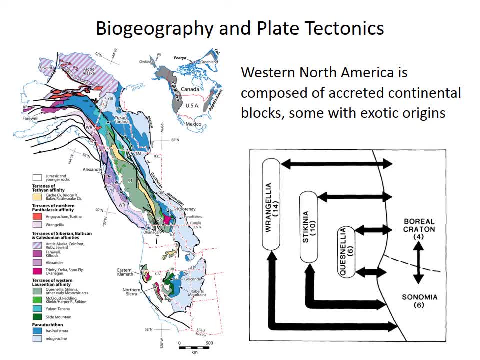 These are called exotic terrains, But the exact locations in which they formed and the movement and timing of their attachment to North America are uncertain. We can use paleobiogeography to compare the faunal similarity between these terrains and the North American continent. 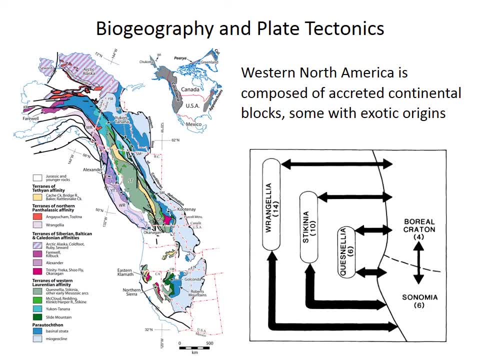 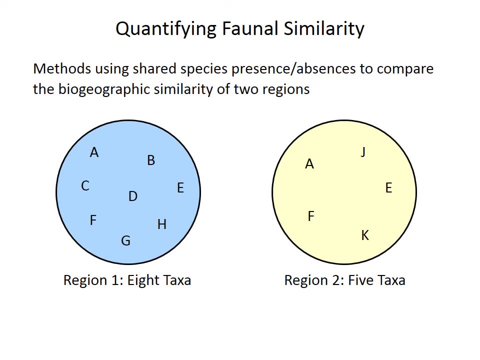 and other continents. but first we actually need to figure out ways to quantify similarity before we can use the faunas to reconstruct movement of these terrains. Methods for quantifying faunal similarity rely on species' presences and absences, as well as shared species between two regions. 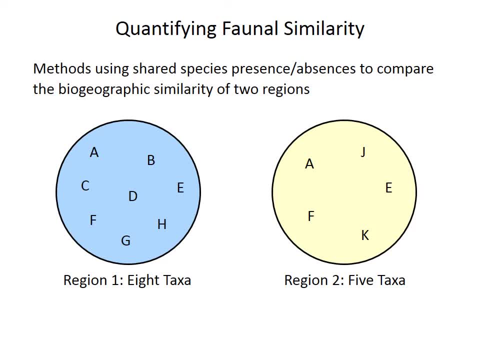 For example, consider these two regions. Region one in blue contains eight taxa letters, A through H, and region two contains five taxa. There are three taxa- E and F- found in both regions and we'll call those shared taxa. For simplicity, we can refer to these as N1 and N2,. 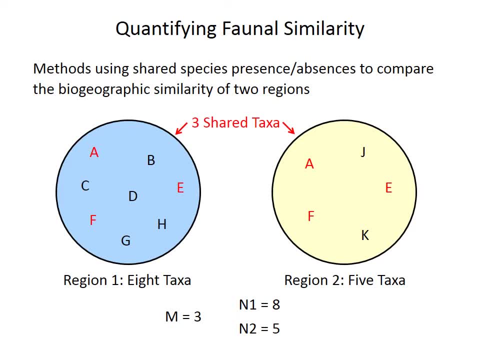 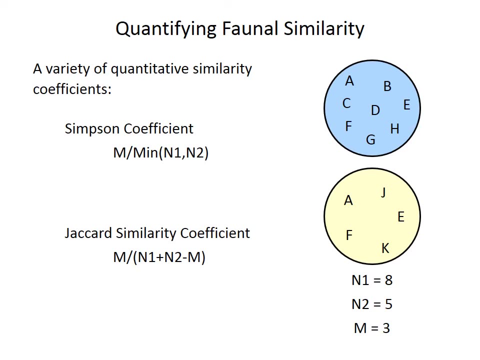 the number of taxa in each region. so N1 is eight for region one, N2 is five for region two and we will call the number of shared taxa M, which is again three. Literally dozens of different similarity coefficients have been proposed over the years. 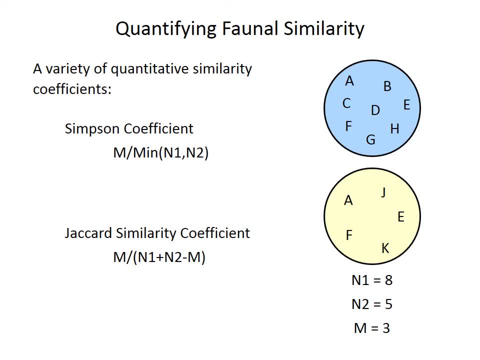 Two widely used ones, although they all have various shortcomings, are the Simpson coefficient and the Jacquard similarity coefficient. The Simpson coefficient is calculated as M, the number of shared taxa divided by the number of taxa found in the smaller of the two regions. 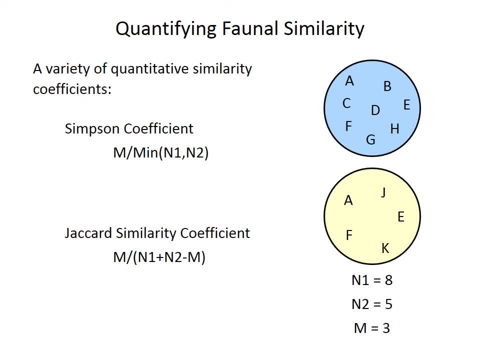 So in our previous example, there are three shared taxa and the smaller region contains five. there are eight in the larger region. therefore, S the Simpson coefficient is just three divided by five or 0.6.. In theory, the Simpson coefficient can vary. 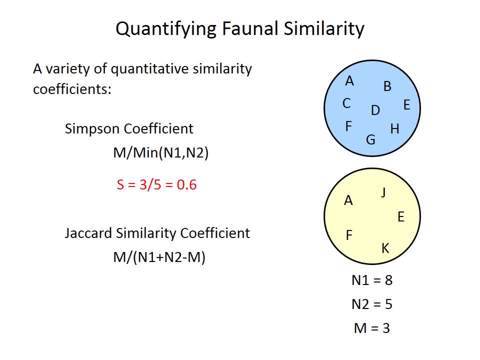 between zero, where there are no shared taxa, or no similarity to one where all the taxa are shared, or we can call that perfect similarity. The Jacquard coefficient is just given as M the number of shared taxa divided by N1 plus N2 minus M. 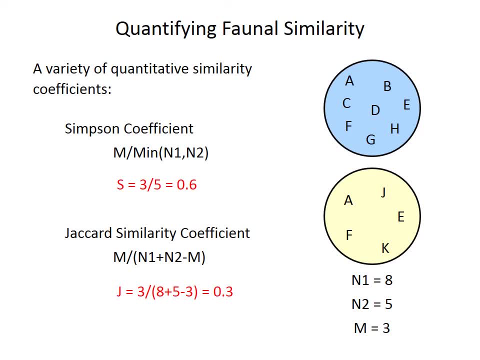 which, in this case, is this: three divided by eight plus five minus three, or 0.3.. The Jacquard coefficient can also, in theory, range between zero and one, but only if the two regions have equal number of species. When one region is smaller. 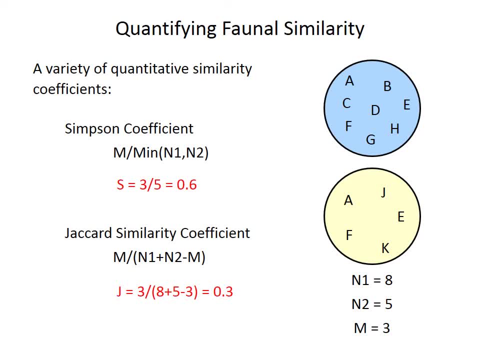 the maximum potential value of the Jacquard coefficient is also reduced. So this is an important thing to consider when interpreting plate tectonic similarity or other interpretations of biogeography. So note that you can't actually compare the actual numbers between different similarity coefficients. 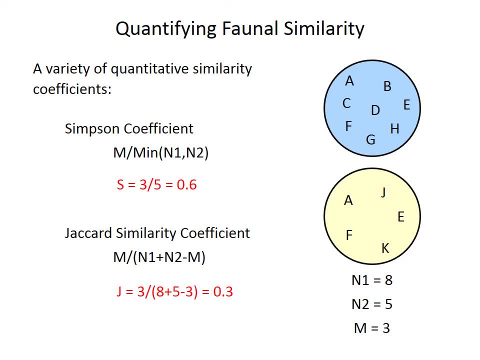 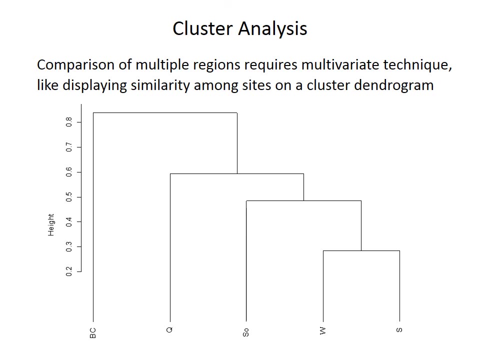 The fact that the Simpson coefficient is 0.6, larger than the Jacquard coefficient is not relevant because they're calculated in very different ways. However, you can compare multiple sites as long as you use the same type of coefficient, But comparison of multiple regions. 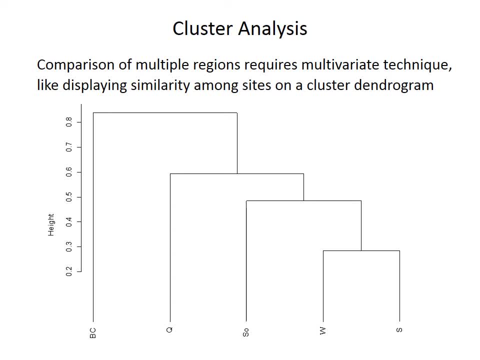 can be complicated because it yields similarity coefficients between all pairs of sites. That can end up being pretty unwieldy if you have more than a few sites. So this example shows five regions and I'll explain the graph in a minute. But with five regions. 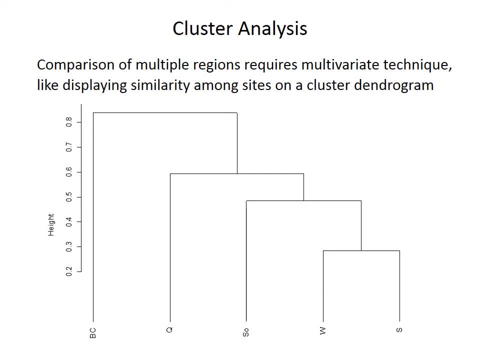 there are 10 possible pairs of sites. If you have 10 regions, there are 45 possible pairs of similarity coefficients And if you have 20 sites, there are 190 pairs. So if you have that many coefficients to examine, you cannot simply just visually determine. 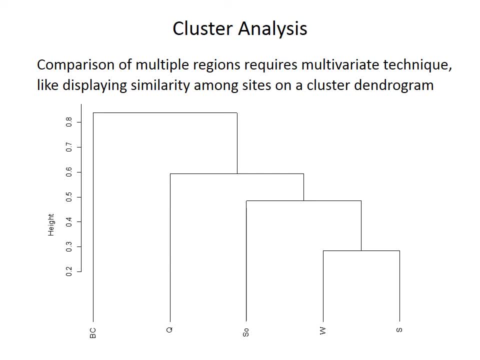 which sites are most similar to each other. So, like before, when we have this complicated multivariate data, we need some sort of technique to analyze these similarities, And for biogeography, cluster analysis is one commonly used method. So this method starts by grouping. 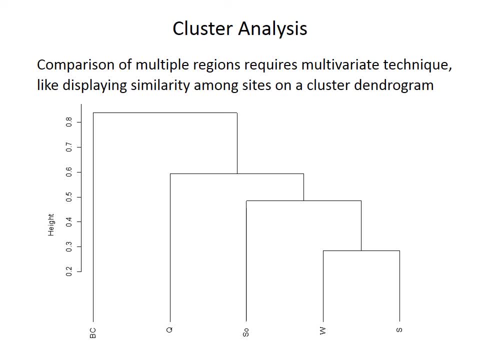 the two most similar sites and then adds additional sites by comparing the average similarity between that site and the ones already in the cluster. In this graph, the y-axis is actually dissimilarity, which is simply one minus similarity, The dendrogram.